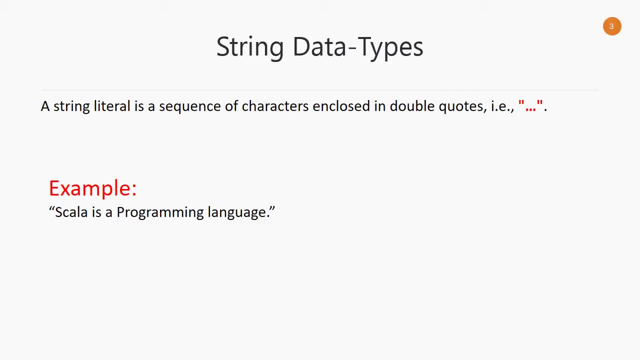 The compiler starts from the first double quote and it tries to find the next one to meet the end of the string. In the next example I have taken a string. Scala is derived from Java. It's more based on functions And I have given a character escape sequence- new line escape sequence- that when the compiler reaches it, it changes it into a new line. 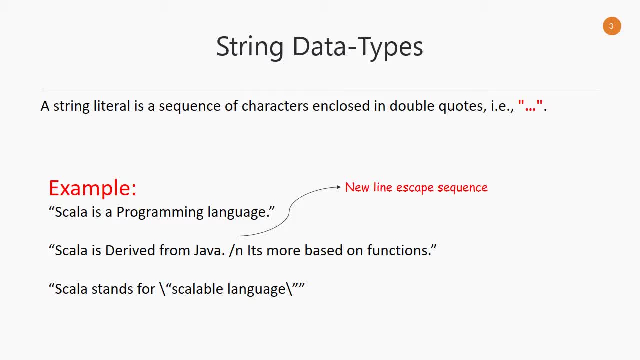 In the third example I have taken a string and I want to give multiple number of double quotes in between them. For that I need to tell the compiler that it is a special character. So we need to assign an escape sequence to detect the double quotes. 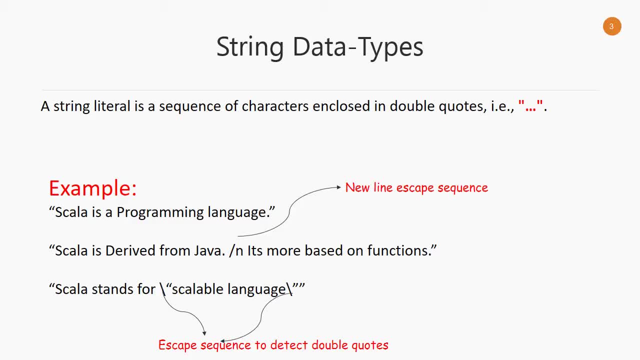 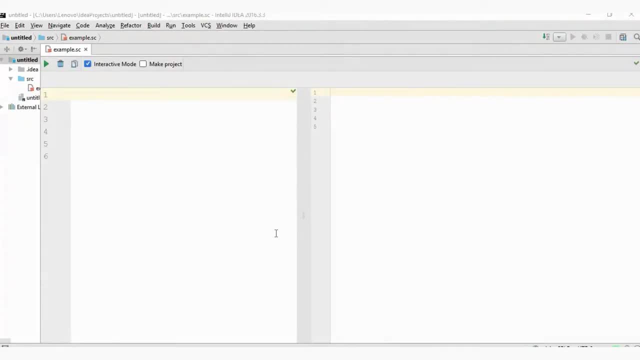 So putting a backward slash in front of double double quote tells the compiler that it is a special character. Let us better understand string datatype in detail. Here I will define a variable named as welcome And I will define it as a string datatype with string. 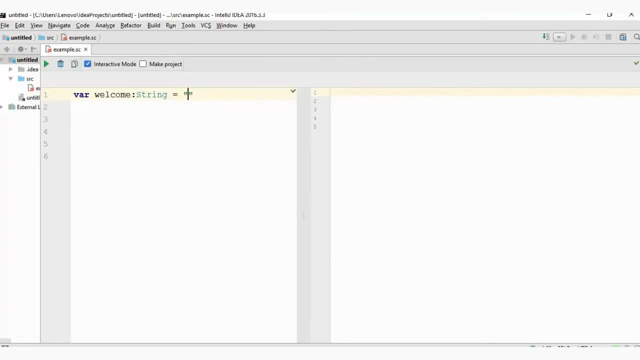 Then I will give the value Hello Scala, So you can see that it is based on REPL concept. So read eval, print and loop. Instantly it gets evaluated and the output is right there. Welcome string. It is string type and hello Scala is the message. 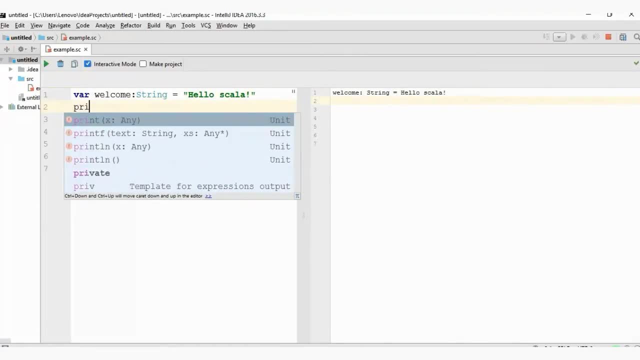 And if I try to print the variable, So I should write print ln and in brackets I will write the variable name. that is Welcome. So you should get the output here. You can see the output is hello, Scala. Now let us know about the character escape sequence. 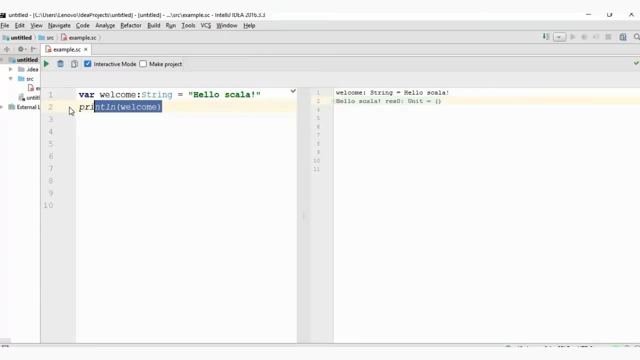 So I will, Let us change it, Hello, and I will put slash and sorry, backward slash and in between them Let us see what is the output. now I will try to print the Variable now Print and print ln. Then in brackets, I will give the variable name. that is welcome.